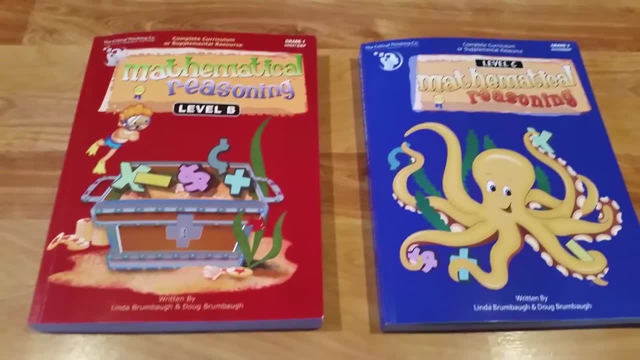 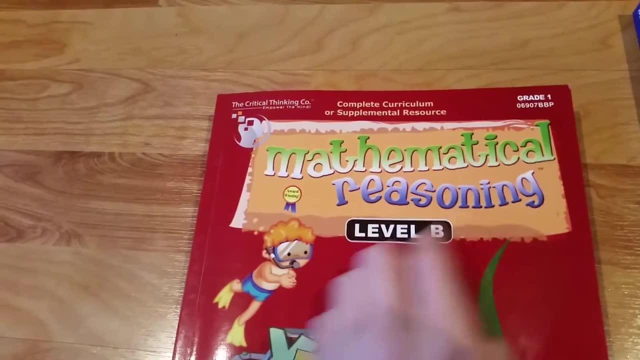 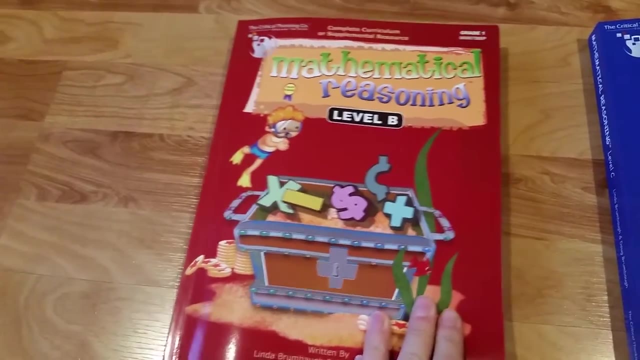 So I'm excited to make one for maybe other people who are looking for that. So for my kindergartner level B, which is kind of equivalent to grade one, I looked at the kindergarten level for him and just thought it was not going to be challenging enough, So we'll jump right in. It has. 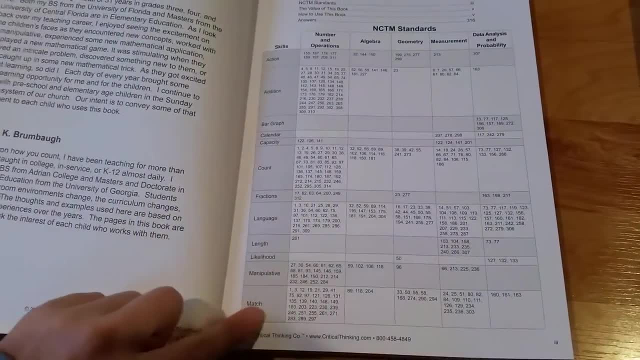 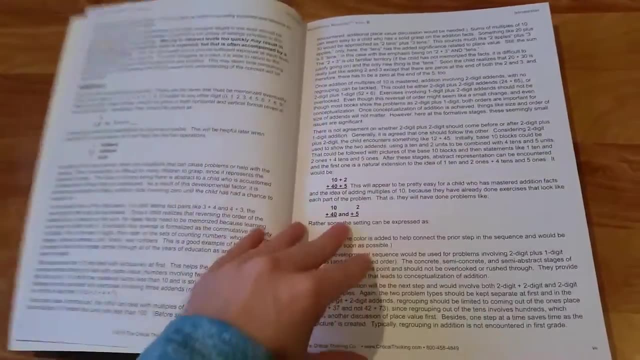 some table of contents that is more just like the concept and what pages that's on. It has some pages how to use the book. It has some pages how to use the book. It has some pages how to use the book, some teaching tips, some just kind of general math reminder type things, And then it just 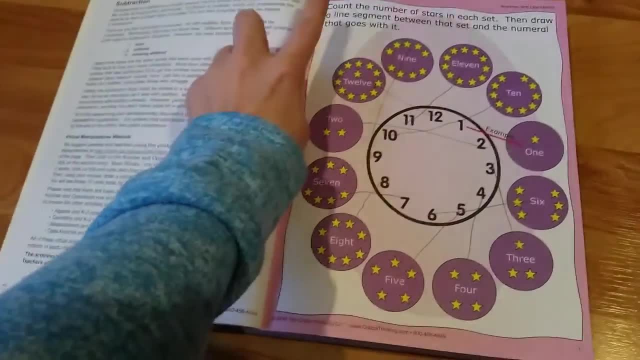 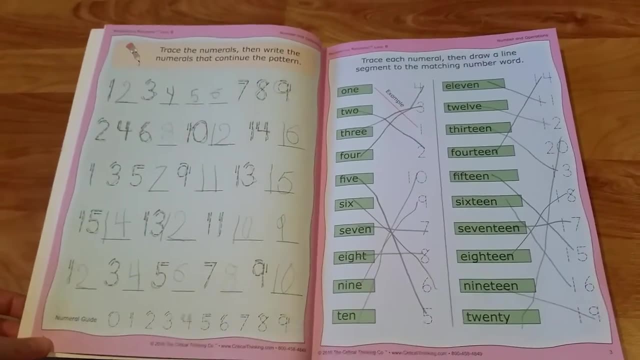 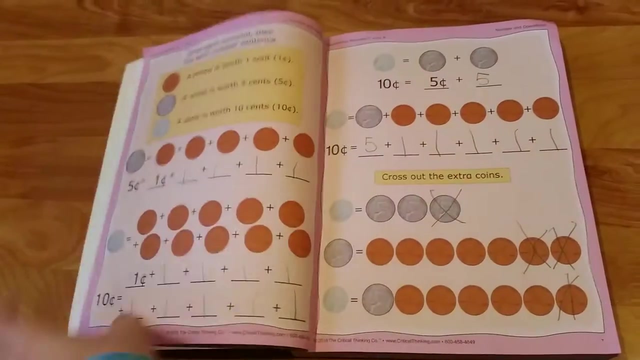 jumped right in. There's no teacher's manual at this. It just gives instructions at the top when needed And just kind of some fun review at the beginning, just filling in the number patterns matching to the number word count the blocks and add them coins Like this one's showing. 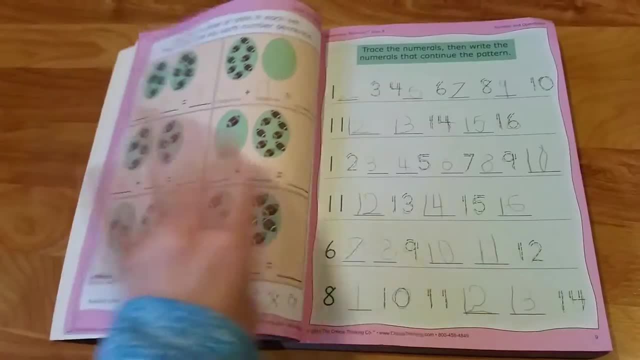 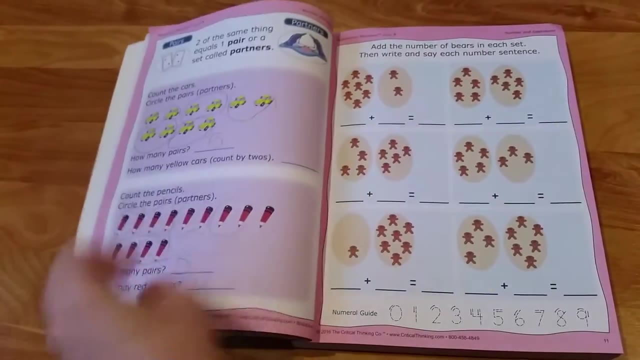 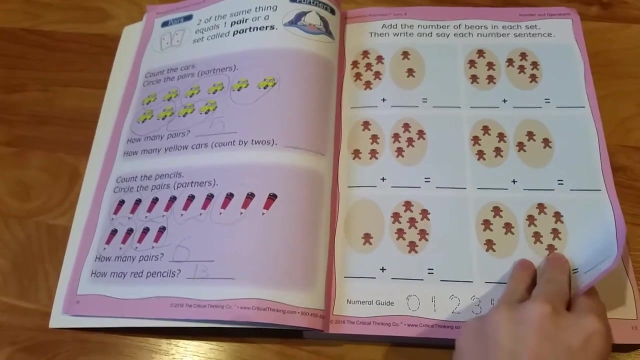 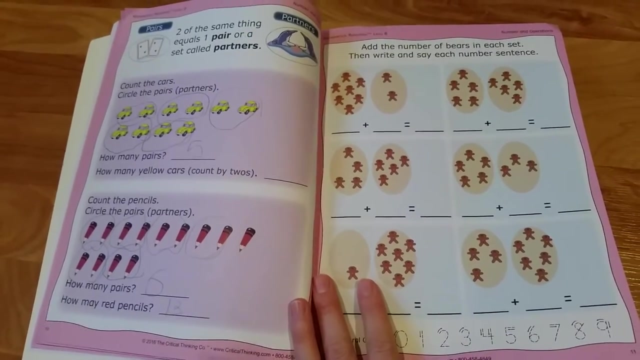 that a nickel is the same as five pennies And it does have some reviews. So here's some more of the filling in the missing number in those number patterns, Pairs and how many pairs are there. How many is that all together? Kind of getting them starting to think about groups and kind of a precursor to 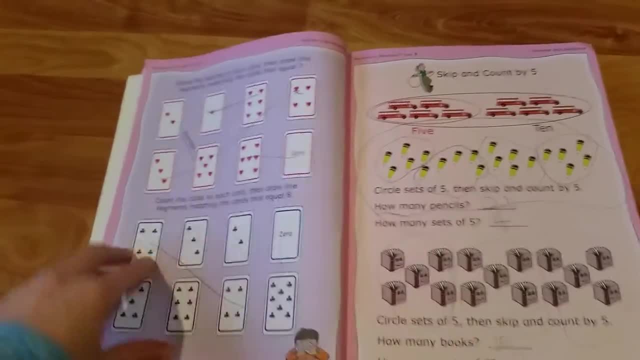 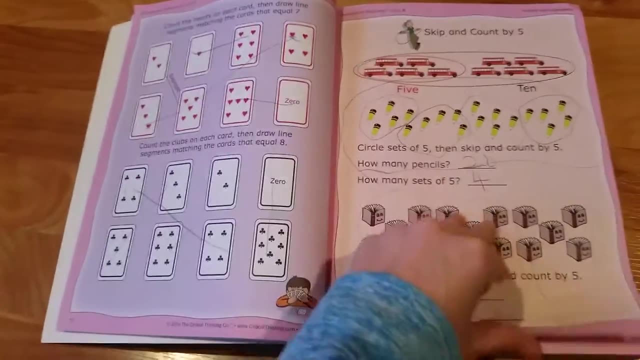 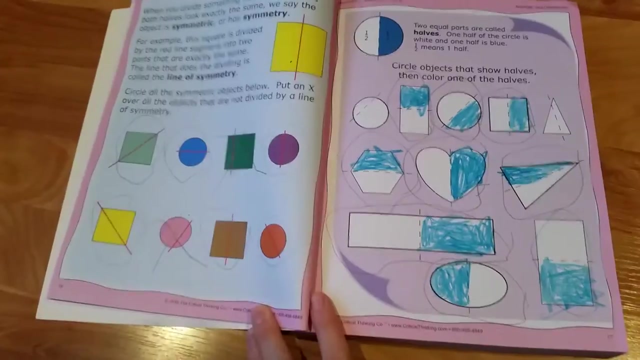 multiplication Match up. This one is: match up the cards that the hearts on them add up to seven More of the groups, And then coins adding, And then when there is a new concept, that isn't something that's pretty self-explanatory. maybe it does have more. 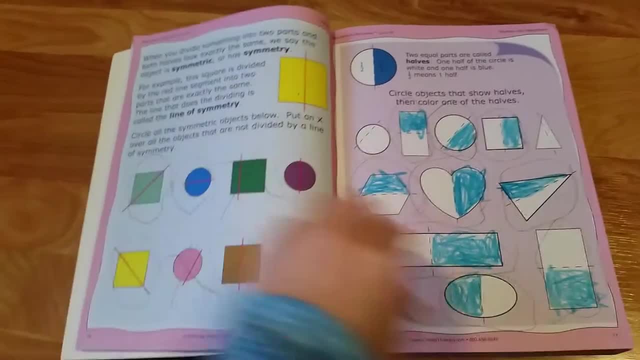 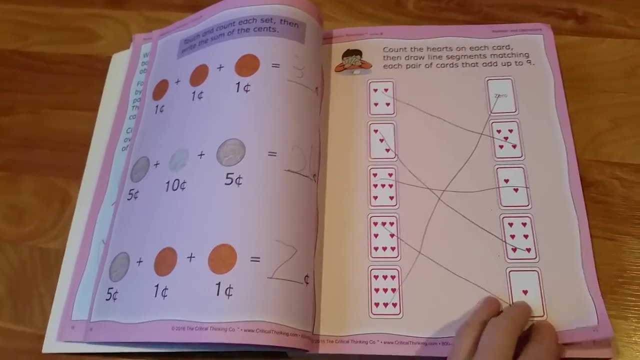 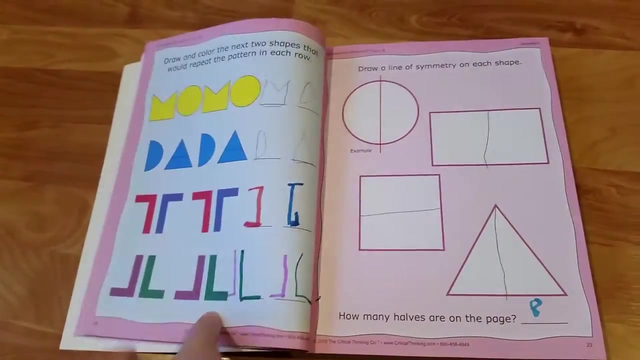 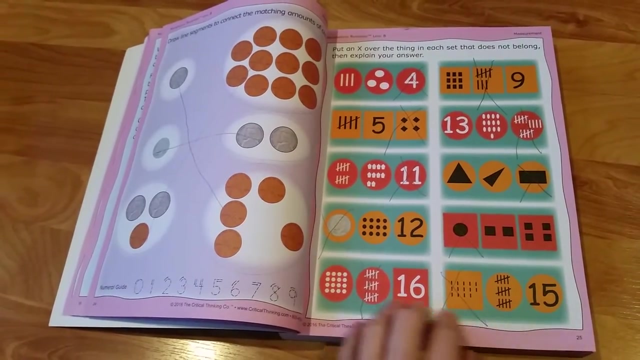 instructions over here. So talking about symmetry And then going back and doing some more similar activities, This time adding up the hearts, add up to nine on the two different cards, Completing patterns. so this is kind of what we've done so far: A little bit of critical thinking, what in? 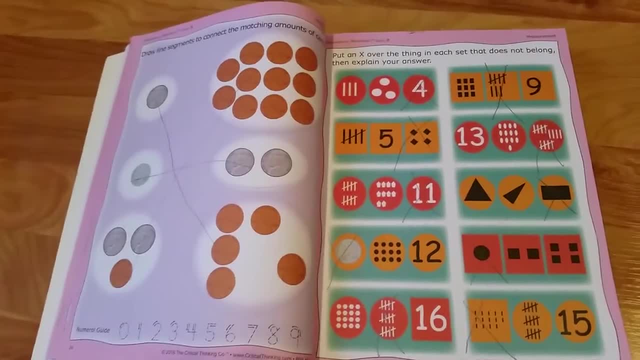 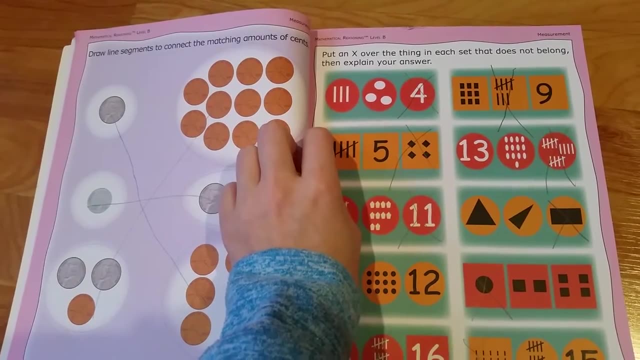 each group doesn't fit, and it was really interesting to hear my son's ideas on these ones. So my younger son is much more creative thinker than my older son, and so he was kind of looking at these and instead of just saying, oh there's. 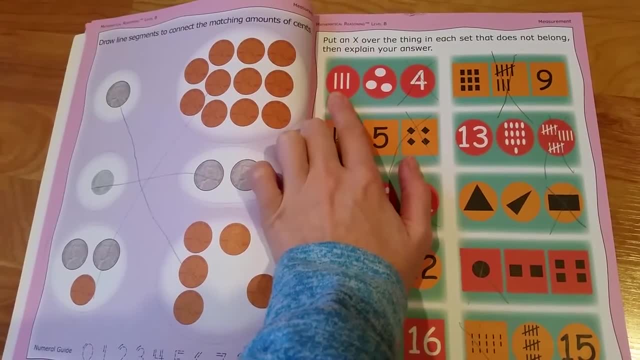 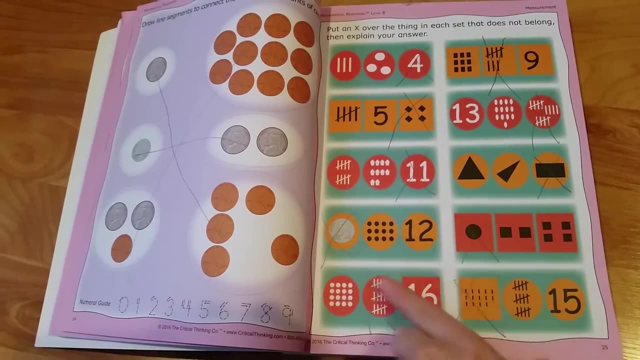 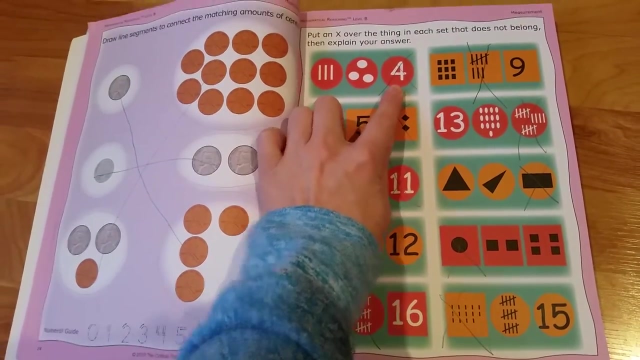 three, three and this is four he was looking at, well, this one is straight lines and this is made of straight lines, or so. it's interesting to hear how he thought about and how he looked at these patterns before coming to the conclusion that it's three, three and this is four, and so that one didn't fit, So going. 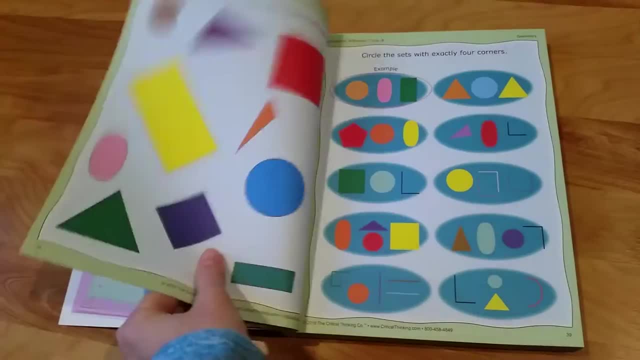 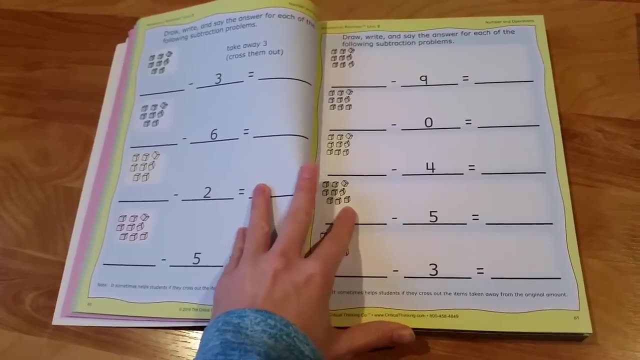 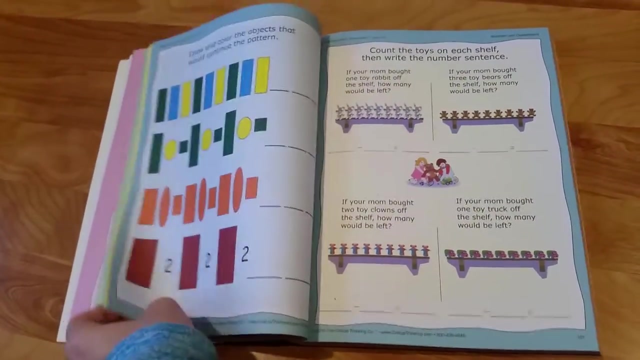 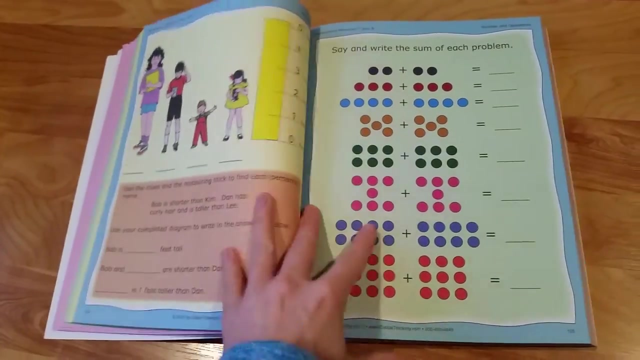 ahead a little bit. there's some number lines and shows them how to add with that What has corners, subtracting, making graphs- I'm skipping quite a bit at a time here, But just very colorful, which my kids really like, and there is quite a. 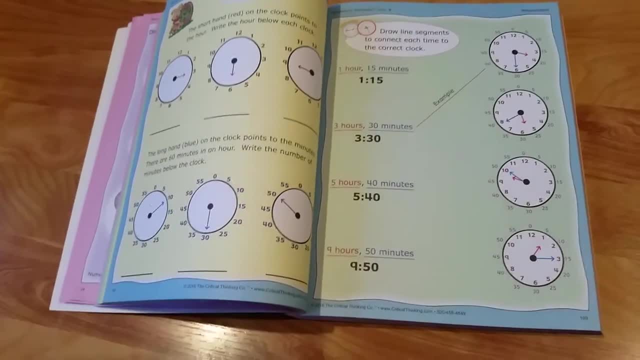 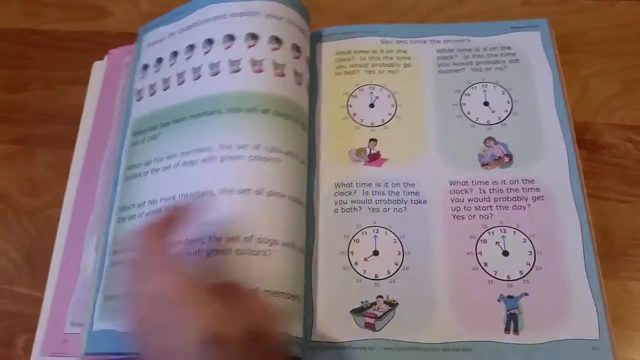 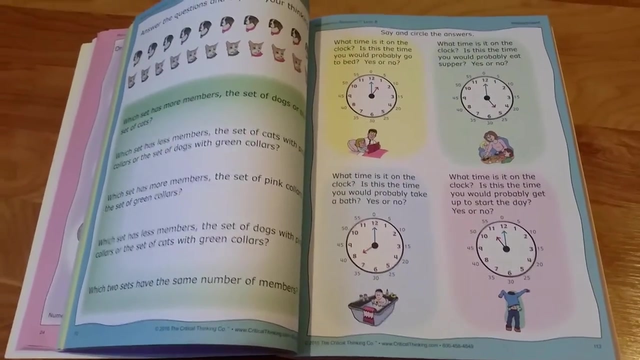 bit of review For my kindergartner. I think these could maybe stand alone for him. Some people use these as standalone curriculum. We are using them just sort of as supplement, because my kindergartner is probably about three-quarters of the way through our Saxon math and it's we're only about a third of the way. 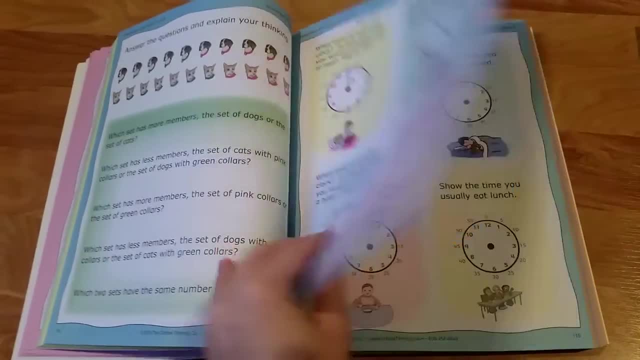 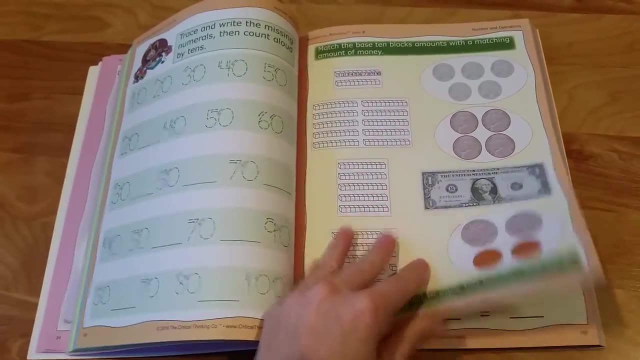 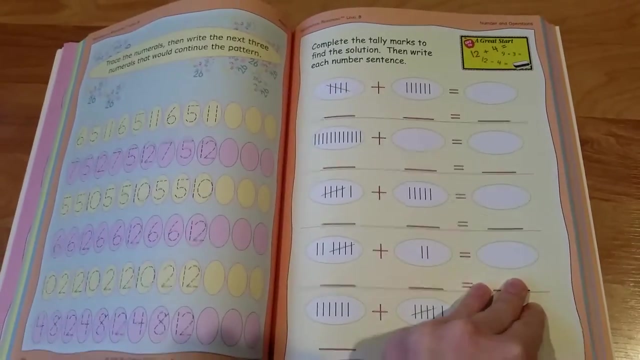 maybe half, maybe half the way through the year really. So he is flying through the math, So this is good for him to have extra. So just a good peek inside. and these are separated So you'll notice the pages are different colors, So they're. 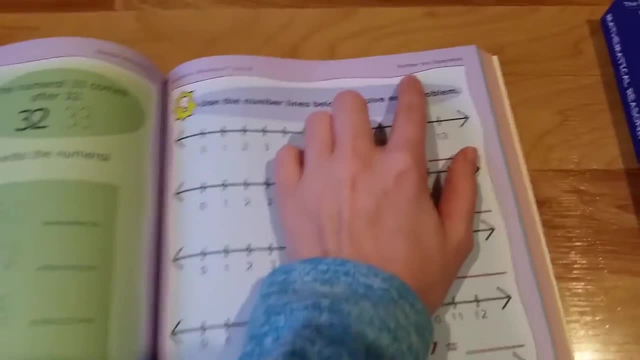 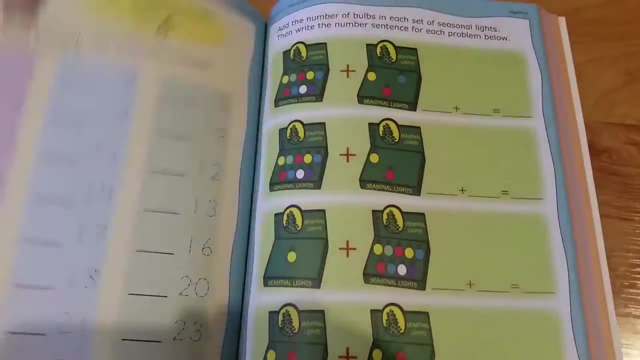 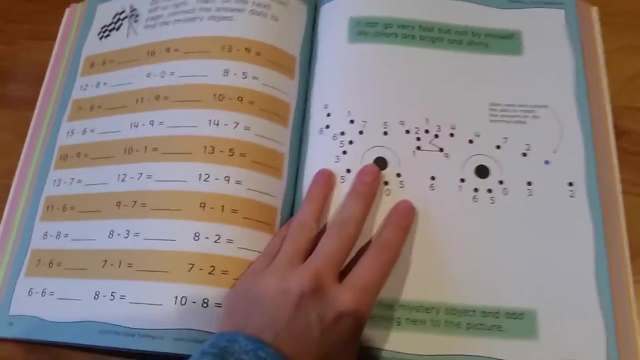 kind of separated into sections and then the top of the page it says what they're working on. So number operations and then let's see algebra, What else. These are fun. My older son has done these in his book already, but it's a dot-to-dot, but it's kind of fun to use. 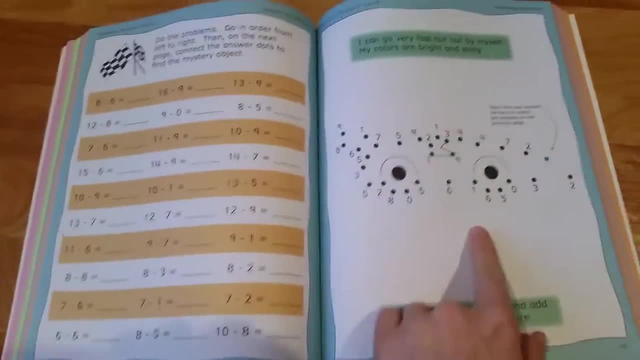 and then these are fun. my older son has done these in his book already, but it's a dot-to-dot. but it's a dot-to-dot. it doesn't go in order like a typical dot-to-dot, They first have to answer the questions over here. 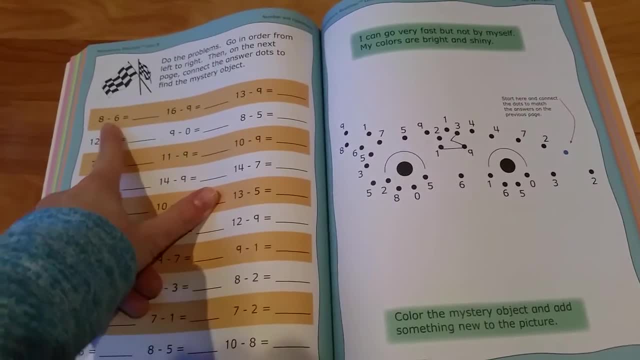 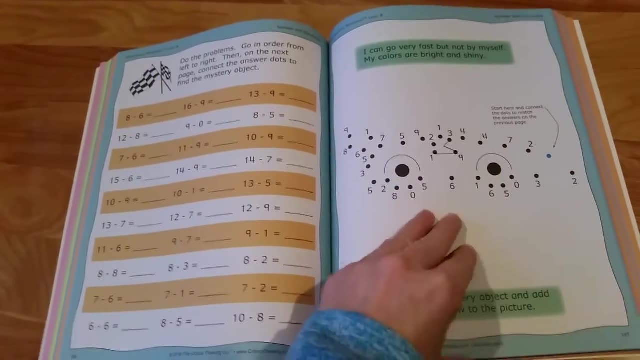 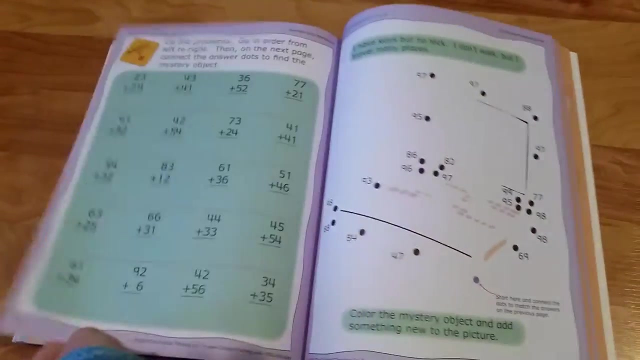 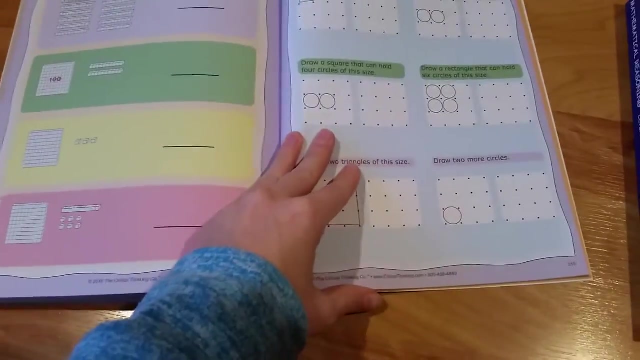 and then, whatever the answer is, it tells them where to start and then, whatever the answer is, they go in order with their answers to form the picture. So that's kind of a peek inside the level B or kind of equivalent to first grade level. and then there are in the very back, there is answer key. Let me show you that. 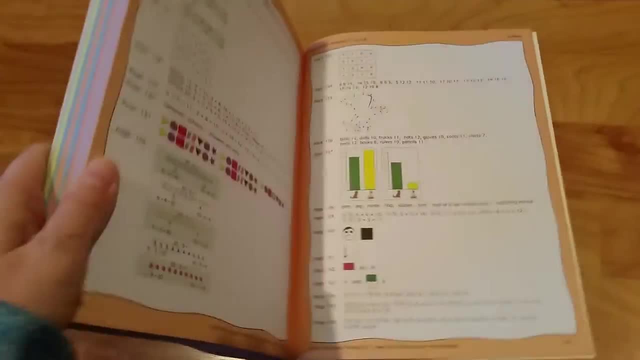 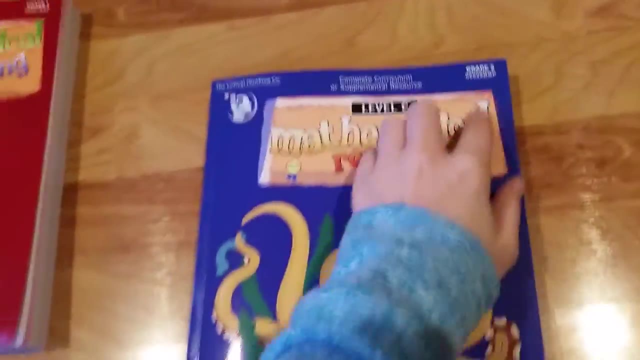 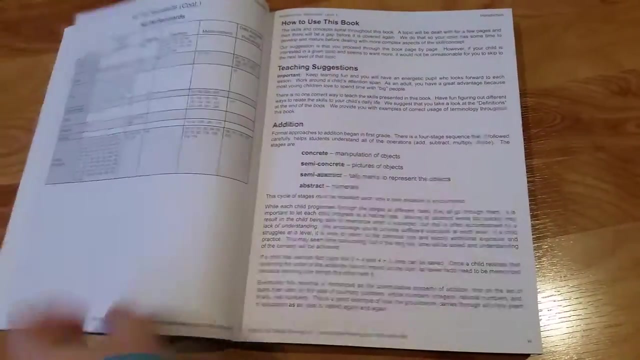 if you need it. Most of these at this level we probably don't, but it is there in case there is a question on that. So that was level B, and then this is level C or grade two that my second grade son is using. Again, it has table of contents and some little bit for 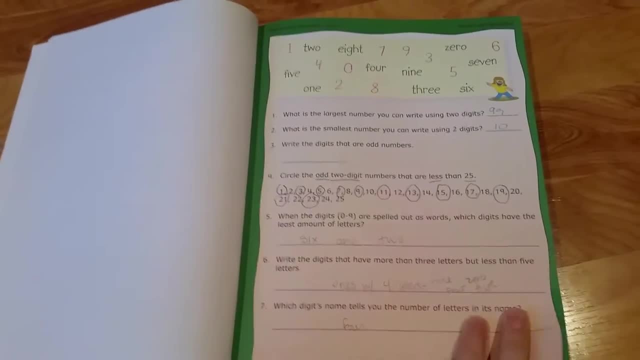 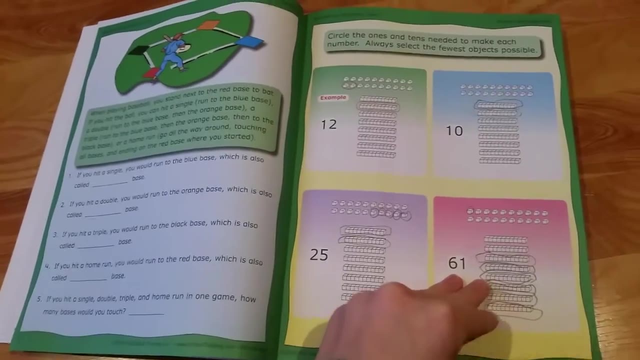 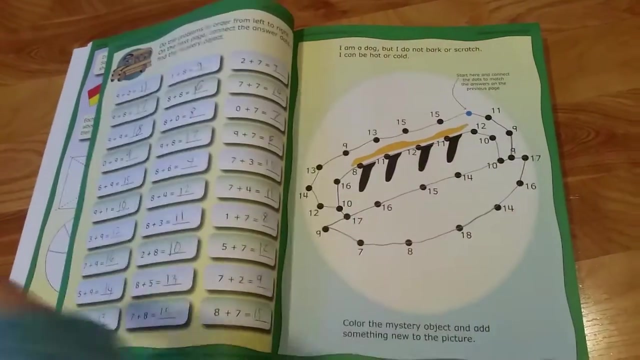 teaching Teacher or parent and then kind of jumps right in. He did this. he just didn't write down the answers because he was too excited to get going and just answer them And just has a lot of these things are. I feel like they match up really well with what he is learning in Saxon 3 and it's a good 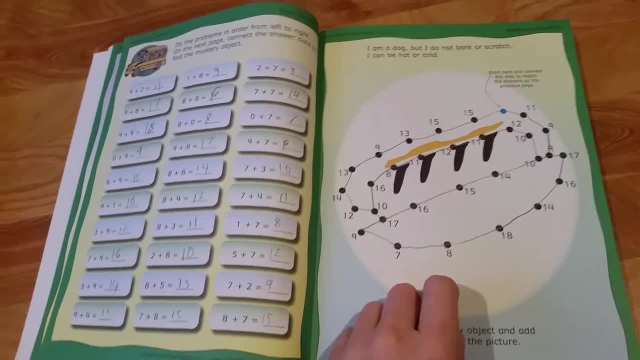 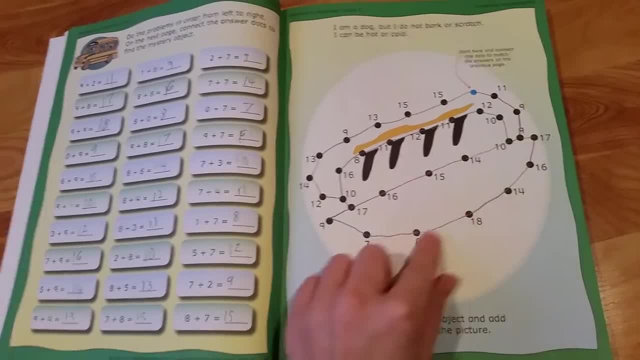 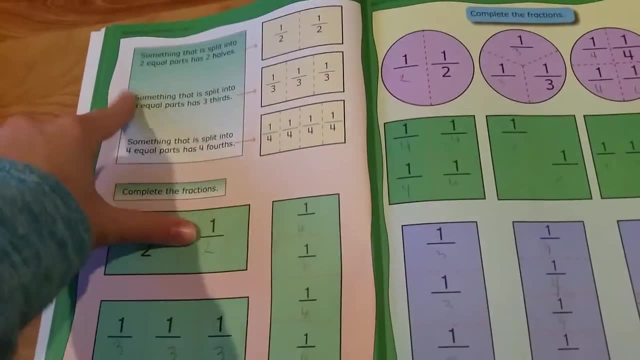 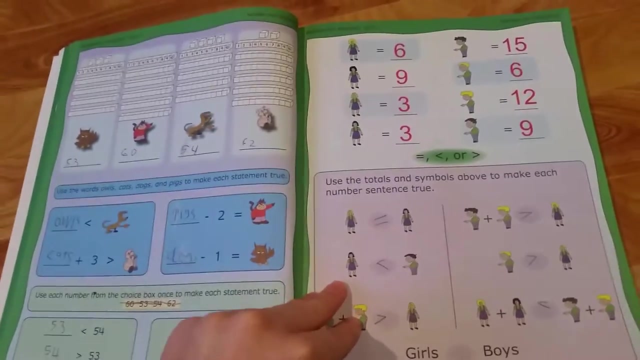 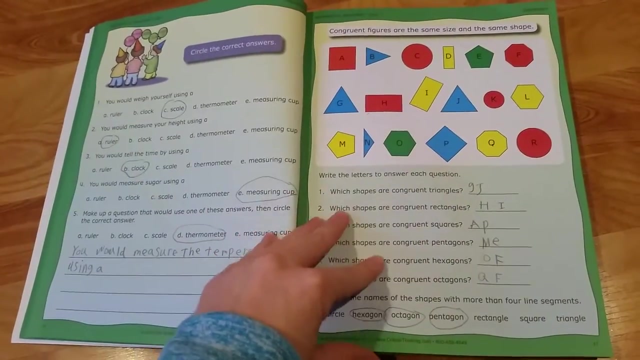 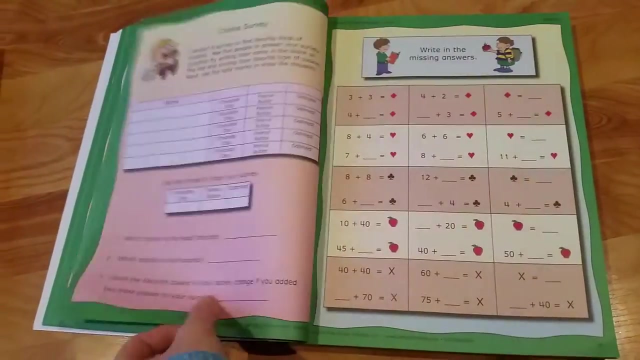 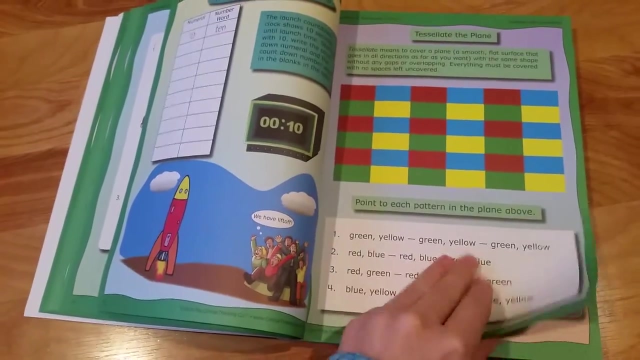 from left to right to complete the dot to dot fractions and it does a little bit of explanation over here and then he filled in the fractions less than, equal to greater than, and so it does have some review kind of spiral as they are going through it and I feel like this is challenging enough for him that, but it's also fun and interesting enough. he my 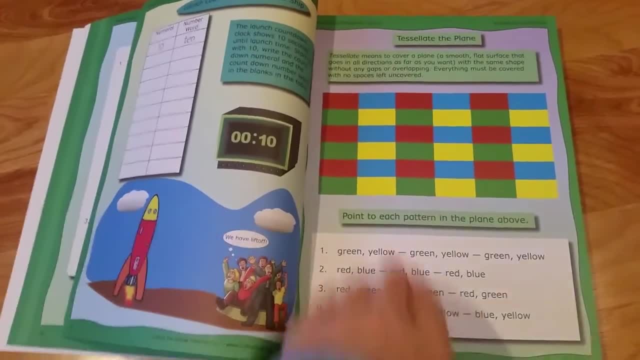 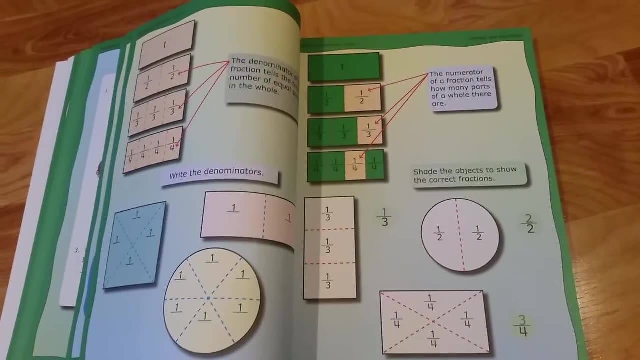 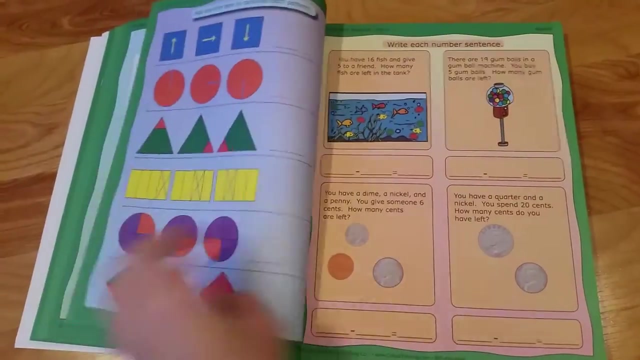 older son is not, as I guess he is much more the type that needs the Saxon match math teachers manual that is very explicit in its instructions and very step-by-step, and then he is good. I am not sure that these books would work for him as a standalone curriculum. 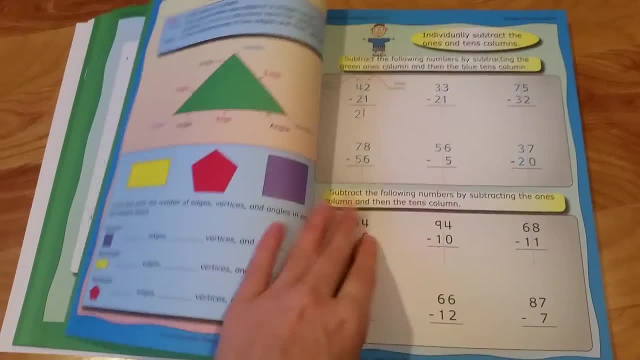 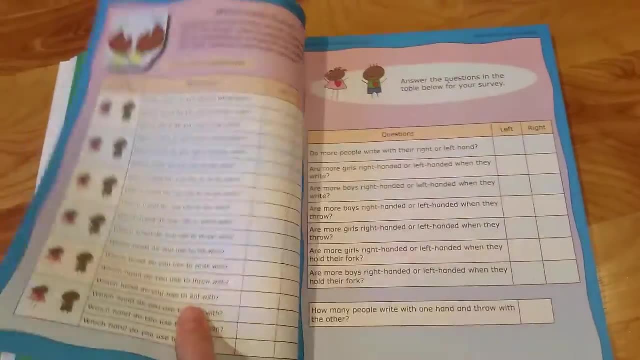 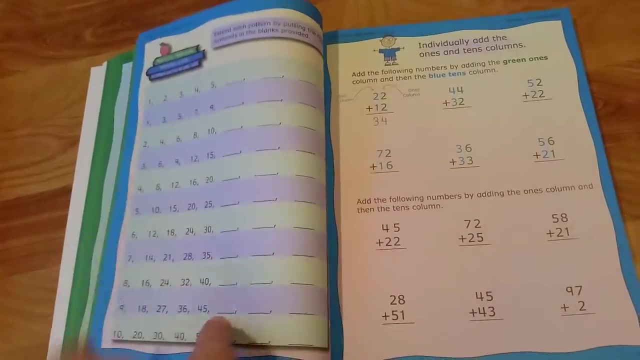 because they may not have quite enough instruction for him, but he does really enjoy so far, Just kind of having the fun extras. So I'll just show you a few more activities like this is a survey and then they fill out, answer the questions and lots of.